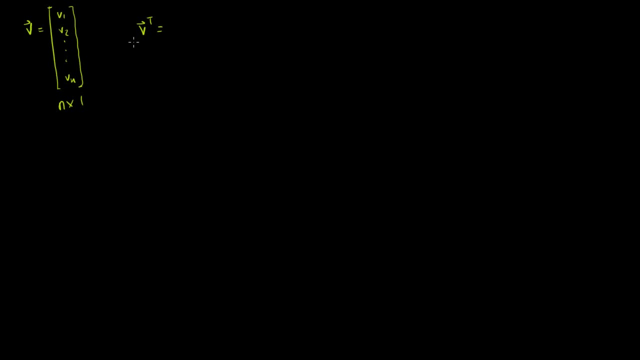 it has n rows and 1 column. then what are we going to get? We're going to have a 1 by n matrix when you take the transpose of it, And this 1 column is going to turn into the 1 row. 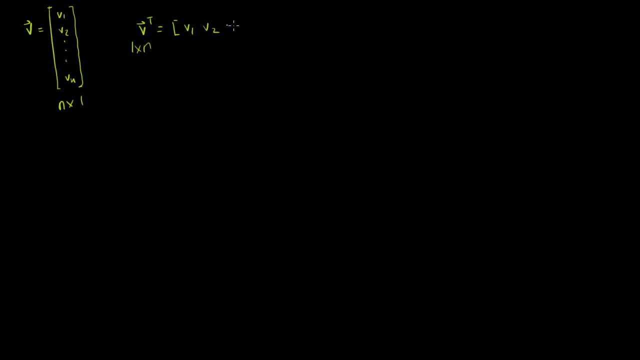 So you're going to have it be equal to v1, v2, all the way to vn, And you might remember we've already touched on this in a lot of matrices before. Let's say that's some matrix A. We called the row vectors of those matrix. we called them. 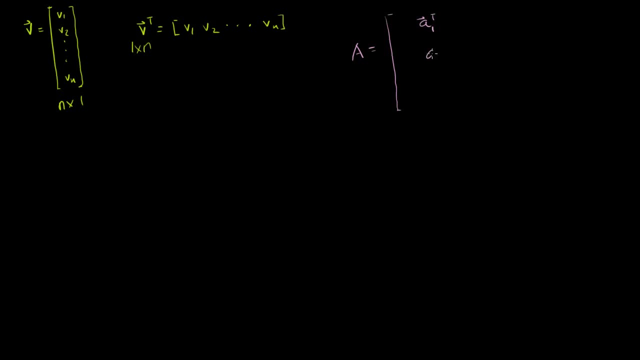 the transpose of some column vectors: A transpose, a1, transpose, a2, transpose, all the way down to an transpose. In fact, not so many videos ago I had those row vectors And I could have just called them the transpose of column. 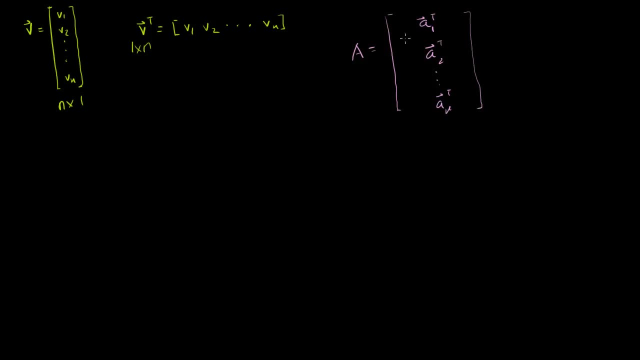 vectors just like that. And that would have been in some ways a better way to do it, because we've defined all these operations around column vectors so you could always refer to the transpose of the transpose and then do some operations on them. 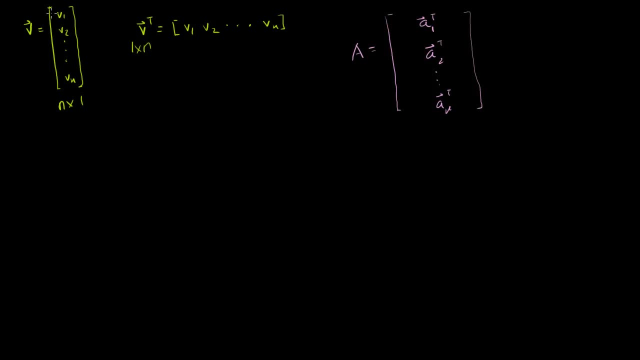 But anyway, I don't want to get too diverted. but let's think a little bit of what happens when you operate this vector or you take some operation of this vector with some other vectors. So let's say I have another vector here, that's w and it's 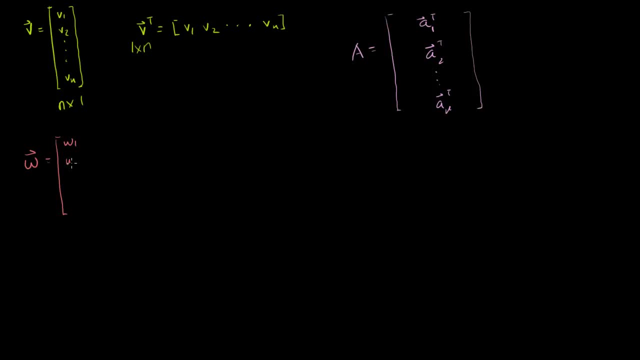 also a member of Rn, So you have w1, w2, all the way down to wn. There's a couple of things that we're already, I think, reasonably familiar with. You could take the dot product of v and w. 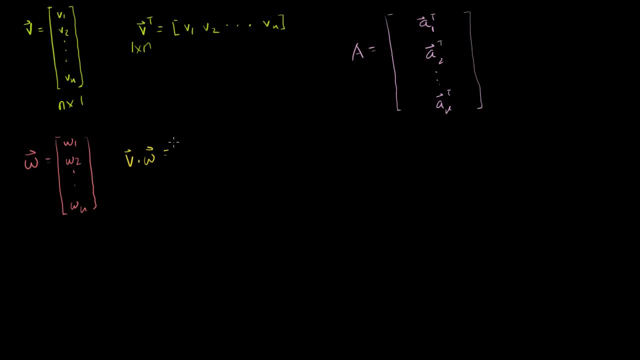 v dot w is equal to what. It is equal to v1 times w1 plus v2w2 plus v2w2, and you just keep going all the way to vnwn. This is the definition of the dot product of two column vectors. 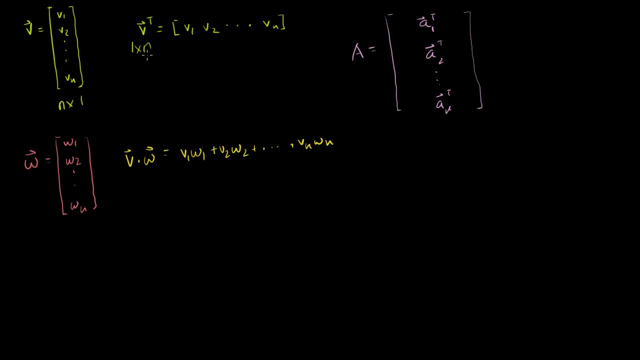 Now, how can we relate that to? maybe the transpose of v? Well, we could take the transpose of v. Let me write it this way: What is if I did a matrix multiplication? so I did v1,, v2, all the way to vn. so this is v transpose. 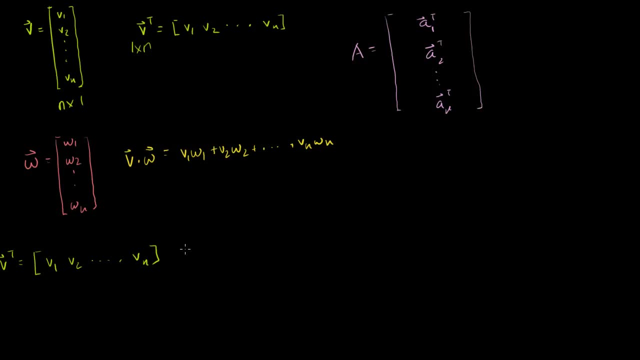 That's v transpose, and I take the product of that with w. I take the product of that with w, So I have w1, w2, all the way down to wn. Now, if I view these as just matrices, this: 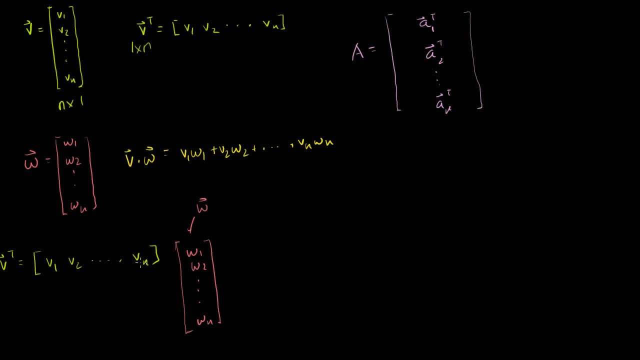 is w right here If I viewed these just as matrices. is this matrix, matrix, point Product well-defined? Over here I have a n by 1 matrix. Sorry, here the first one I have is a 1 by n matrix. 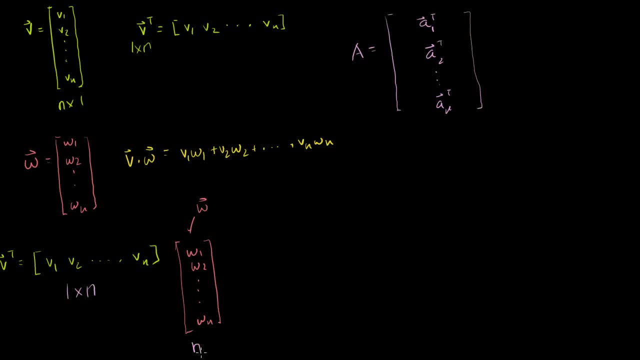 I have one row and n columns, And here I have an n by 1 matrix. I have n rows and only one column. So this is well-defined. I have the same number of columns here as I have rows here, And I'm going to 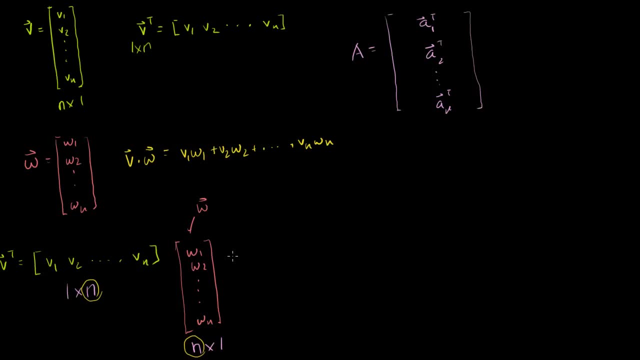 This is going to result. This is going to result in a 1 by 1 matrix, And what's it going to look like? It's going to be equal to v1 times w1.. Let me write it like this: v1, w1, plus v2, w2.. 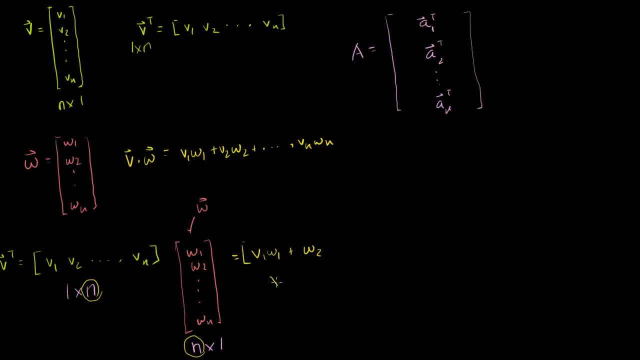 It's only going to have one entry. We could write it as just a 1 by 1 matrix, like that. Let me just do it 1 by 1 matrix, like that: v1, w1, plus v2, w2.. 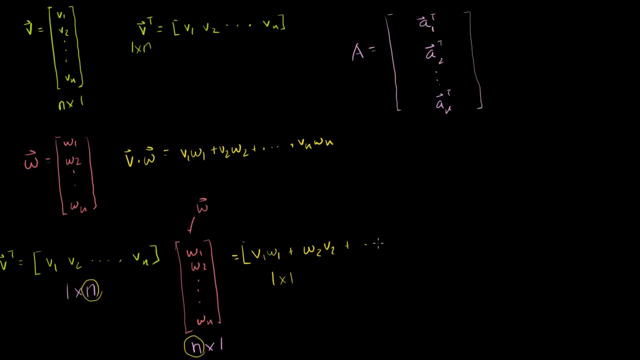 Let me just I could write v2 there Plus All the way to vn, wn. That's what it'll be. It'll just be a 1 by 1 matrix that looks like that, But you might notice that these two things are equivalent. 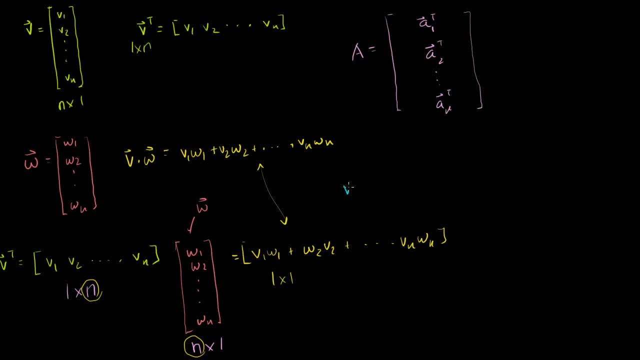 So we can make the statement that v dot w, which is the same thing as w dot d, These things are equivalent to. v dot. w is the equivalent of- Let me just write it once over here: v dot w. v dot w is the same thing as the transpose of v times w, as. 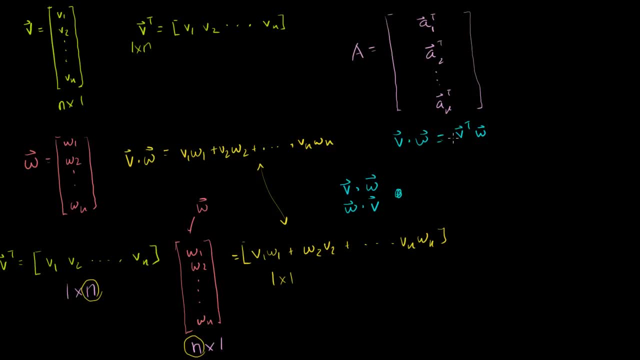 just a matrix-matrix product. So if you view v as a matrix, take its transpose and then just take that matrix and take the product of that with w. it's the same thing as v dot w. So that's an interesting takeaway. 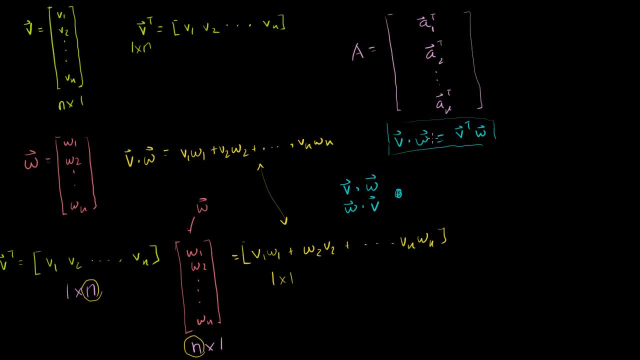 I guess you could argue somewhat obvious, And we've already been referring this. When I define matrix-matrix products, I kind of said you're taking the dot product. It's the dot product of each row with each column, And you can see that it really is. 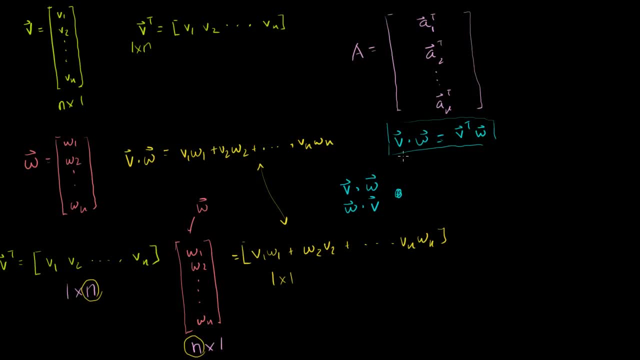 It's really the dot product of the transpose of that row with each column. But you've got the general idea. But let's see if we can build on this a little bit. Let's say I have some. let's say I have some. matrix A: 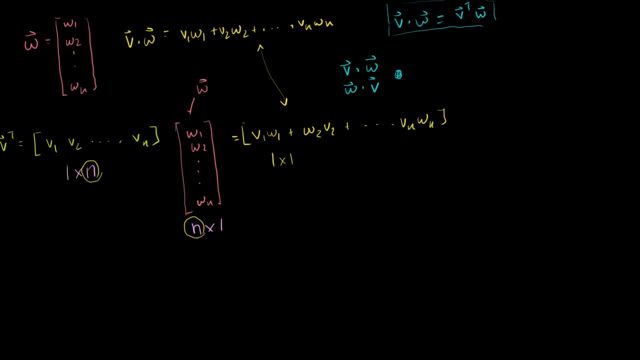 Let me save our little outcome that I have there. Let's say I have some. let me get a good color here. Let's say I have some matrix A and it's an m by n matrix. If I were to multiply that times a vector x, so I'm going. 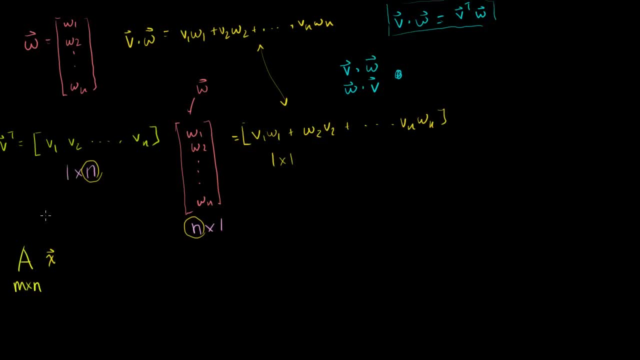 to multiply it by some vector x. Let's say that x is a member of Rn, So it has n elements. Or another way you could view it is: it's an n by 1 matrix. Now, when I take the product of these, what am I going to? 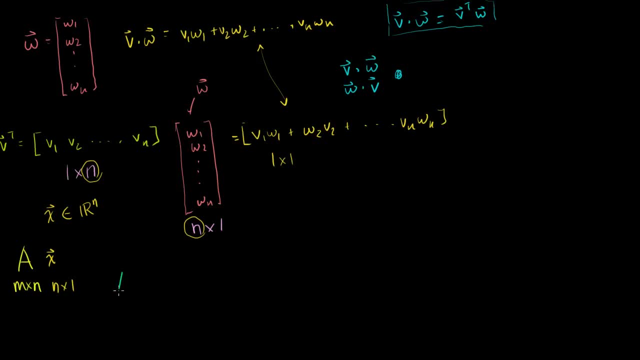 get, Or another way to say it is: what is the vector? ax? When I take this product, I'm just going to get another vector and what's it going to be? It's going to be an m by 1 vector, So we could say that ax is a member of Rm. 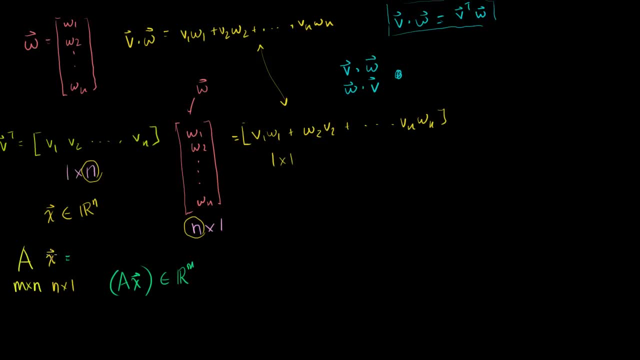 It's going to have m elements, right. If you said that ax is equal to I don't know, let's say it's equal to z, z would have m elements. You would have rm, Right, have z1,, z2, all the way down to zm. 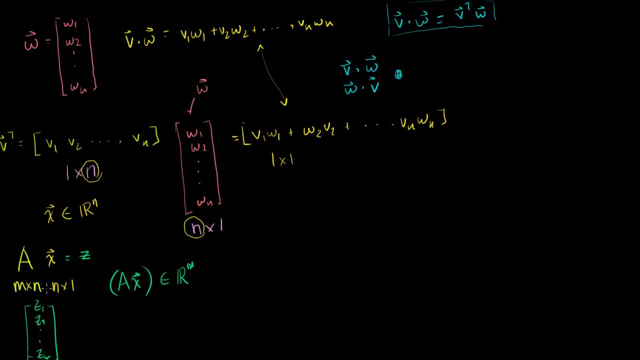 And I know that because you have m rows in A and you have only one. well, you could say: this is m by n, this is n by 1.. The resulting product will be m by 1, or it'll be a vector. 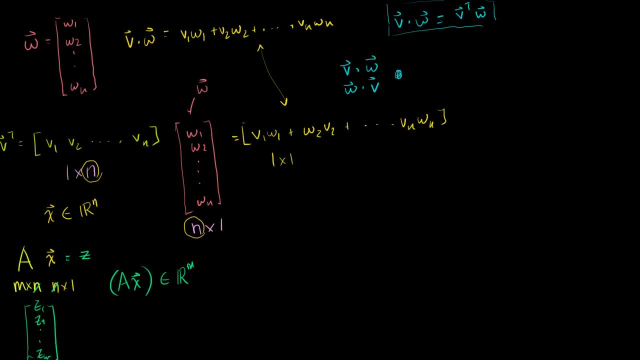 that is a member of Rm, It'll have exactly m elements. Now, if that's a vector of Rm, then the idea of dotting this with another member of Rm is well-defined. So let's say that I have another member of Rm. 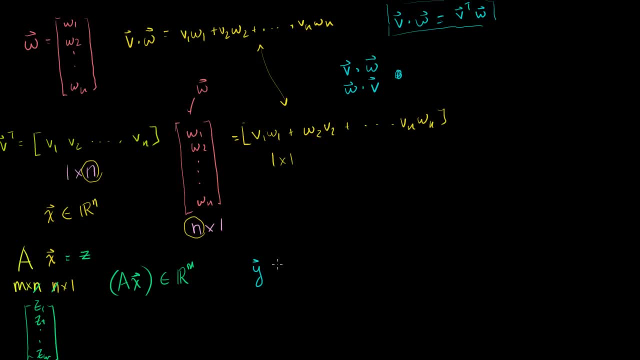 Let's say I have a vector y. Let's say y is also a member of Rm. The vector Ax, the vector that you get when you take this product, has m elements. This has m elements. So the idea of taking their dot product is well-defined. 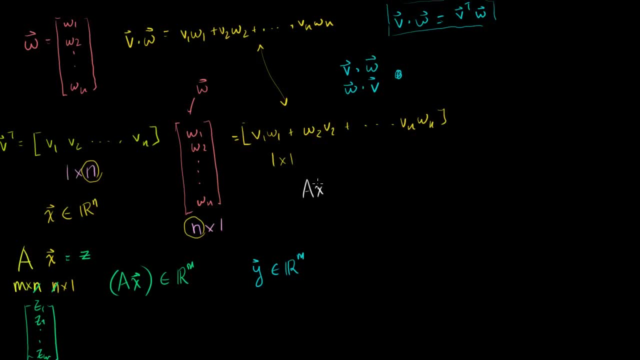 Let me write that. So we could take Ax, that's a vector, and now we are dotting it with this vector right here And we'll get a number. We just take each of their terms, multiply the corresponding terms, add them all up and you get. 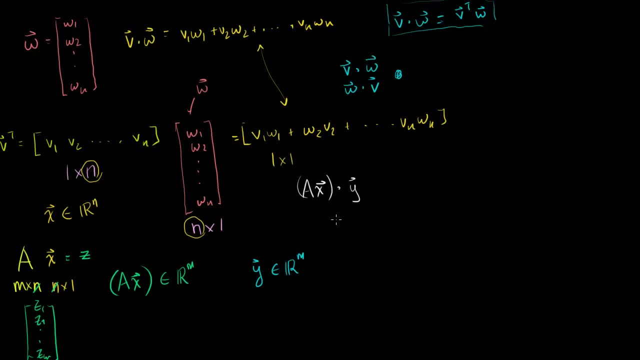 their dot product. But what is this equal to? We can just use this little- I guess you could call it a result that we got earlier on in this video. Using this result, the dot product of two vectors is equal to the transpose of the first vector as kind of a matrix. 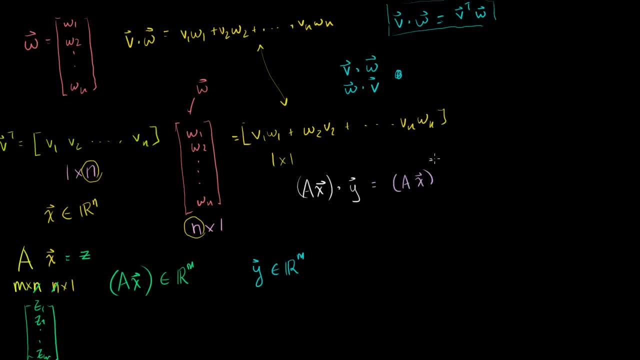 So you can view this as Ax transpose: This is a m by 1.. This is m by 1.. This is m by 1.. Now, this is now a 1 by m matrix. And now we can multiply a 1 by m matrix times y, just like. 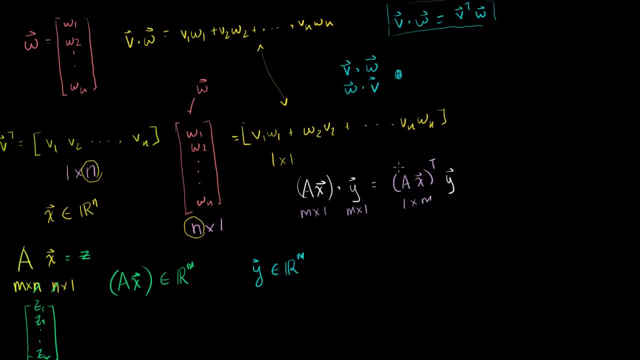 that. Now, what is this thing equal to? We saw a while ago- I think it was two or three videos ago. We saw that if we take the product of two matrices and take its transpose, that's equal to the reverse product of the transposes. 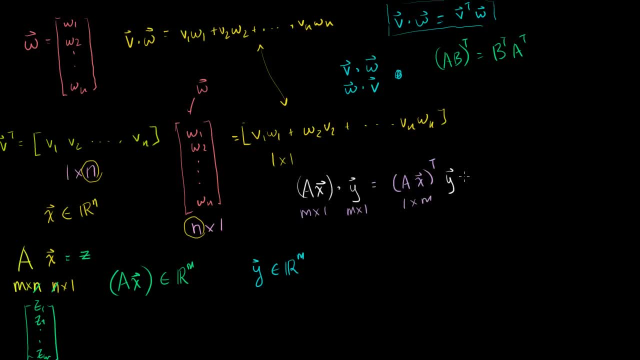 You just switch the order and then take the transposes. So this is going to be equal to this purple part is going to be equal to x transpose times a- transpose times y. This is just matrix products. These are matrix products. These aren't necessarily vector operations. 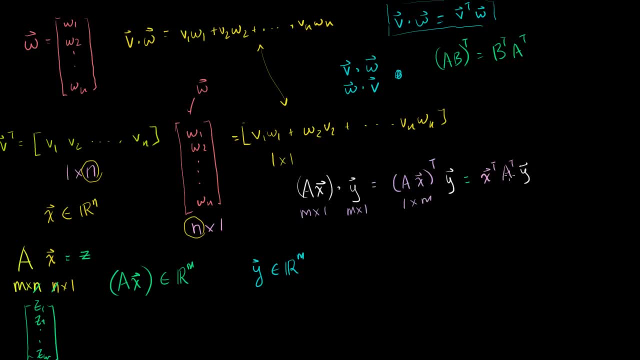 We're treating all of these vectors as matrices And, of course, we're treating the matrix as a matrix. So what is this equal to? Well, we know that matrix products are associative. You could put a parentheses. Right now we have a parentheses around there from: 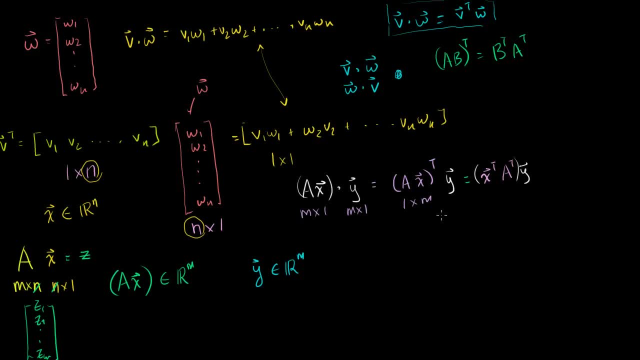 there. but we could just take another association. We could say that that is equal to x, transpose, times these two matrices, times each other. This is a vector, but you can represent it as an m by 1 matrix. so times a, transpose y, just like that. 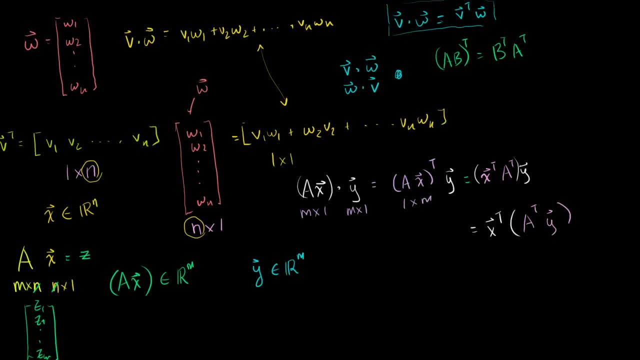 Now let's think about what a transpose y is. Let's think about it. A transpose we have here, a is m by n. What is a transpose? A transpose is going to be n by m, right, It's going to be an n by m. 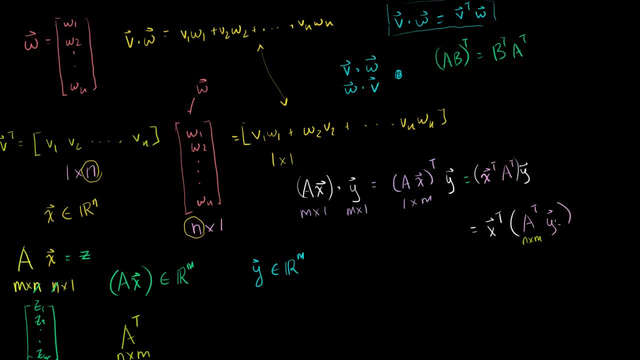 So this is an n by n. And then what is this vector y going to be? This is an m by 1.. So when you take this product, you're going to get an n by 1 matrix, or you could imagine this as a vector that is a. 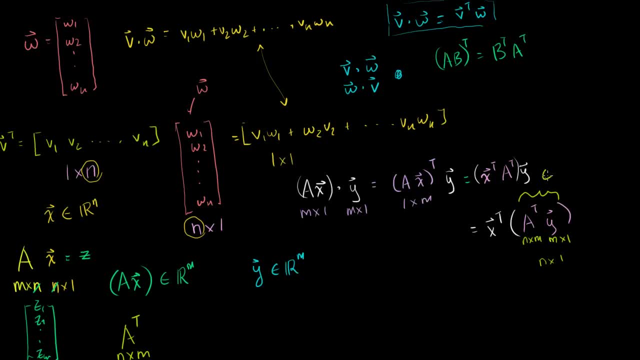 member of Rn. So this is a member of Rn. The entire product is going to result with a vector that's a member of Rn And, of course, it's well-defined because this is a 1 by 1 matrix. 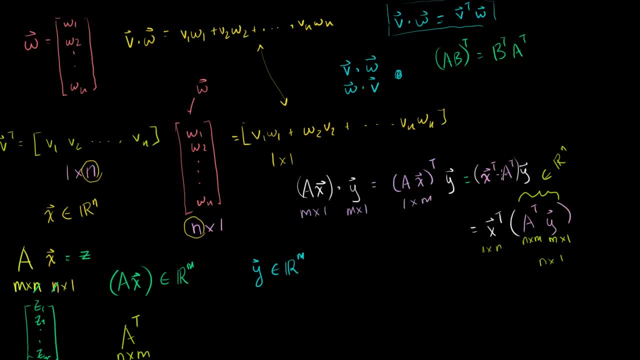 1 by n vector. right there Now we can go back to our identity. We have the transpose of some vector times, some other vector, They have the same. well, I guess you could say this has as many horizontal entries as this guy has vertical entries. 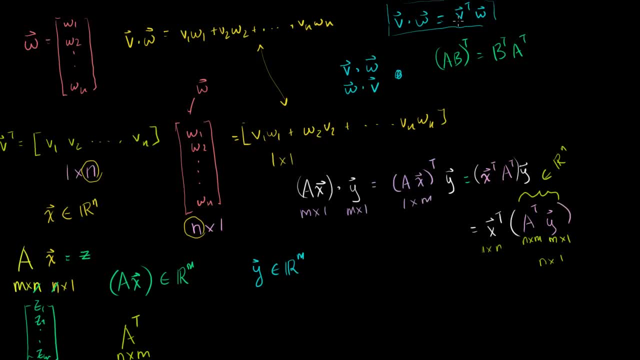 just like that. So what is this equal to? We just use that identity. This is equal to, though, just regular x. in this case, instead of x transpose, we'll just have x. So this is equal to xx. Remember, we just untransposed it. 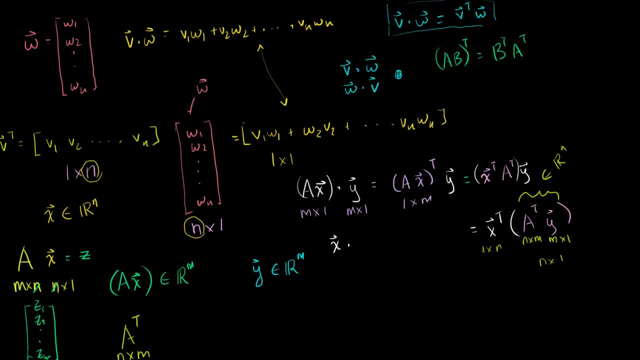 I guess you can view it that way: Dot a, transpose y, which is a pretty neat outcome. We got this. being equal to that, We can kind of change the associativity, although we have to essentially change the order a bit and take the 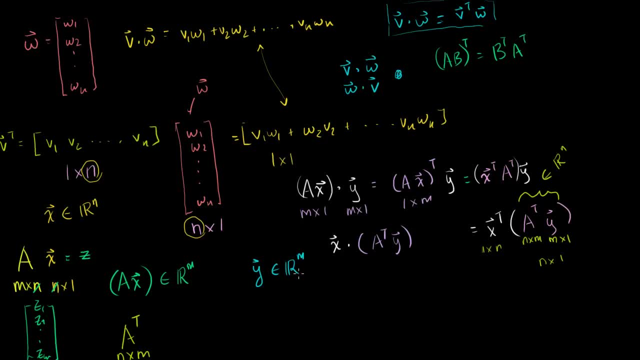 transpose of our matrix. So let me rewrite that just so that you can remember the outcome. So the two big outcomes of this video are- I'll rewrite this one up here: v dot w is equal to the matrix product of v transpose times w. 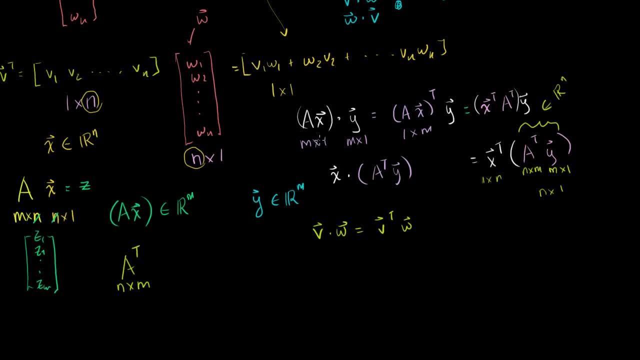 And if I have some matrix, you assume all of these matrix vector products are well-defined and all the dot products are well-defined. If I have ax, dot, y, some other vector y, this is equivalent to. This is equivalent to x dot. you're essentially putting the a with the other.